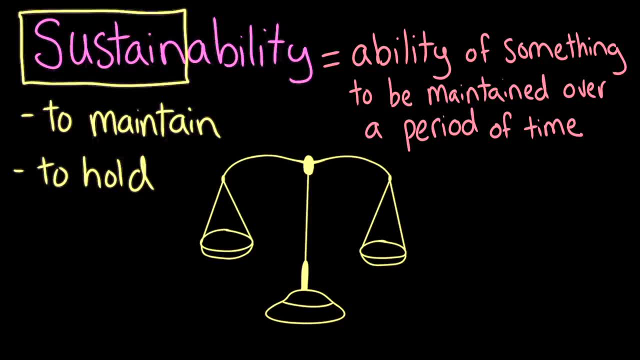 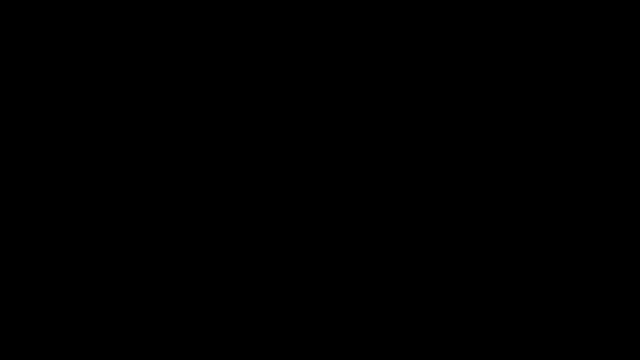 or produce too much So that all the other processes can keep on going, And theoretically, when all these processes are doing their jobs, this balance could last forever, But some things that humans do can disrupt this balance. Let's take a look at an example. In the early years of the United States, enslaved and 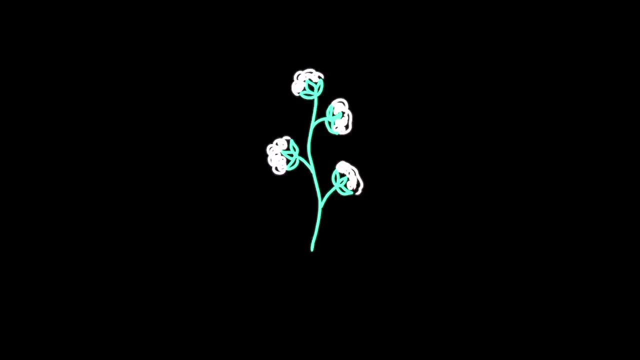 free farm workers in the American South planted, or were forced to plant, cotton, a plant that needs to use the nitrogen in the soil to survive. But when they planted cotton in the same fields, they were forced to use the nitrogen to survive, But when they planted cotton in the same fields, 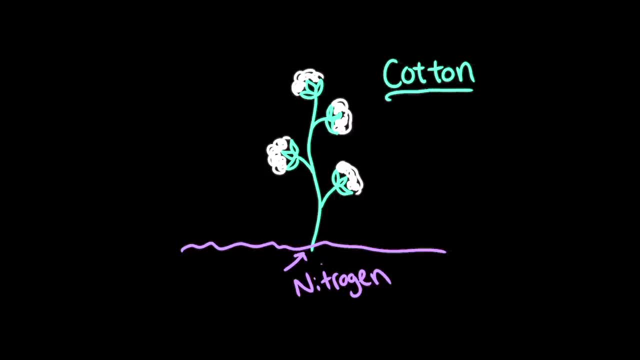 year after year, the cotton plants would deplete the nitrogen levels in the soil. This constant depletion of nitrogen was not sustainable and the cotton crops suffered. In the early 20th century agricultural scientist and inventor George Washington Carver suggested that farmers 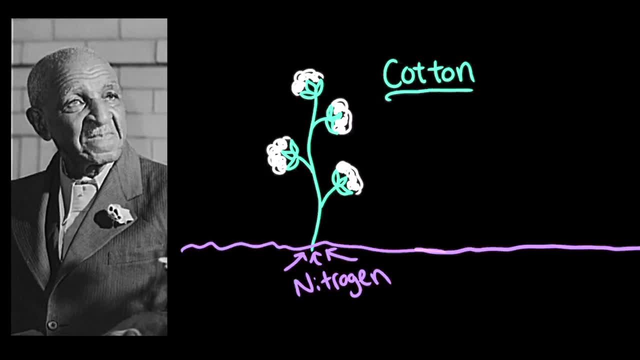 could alternate between growing cotton and growing nitrogen-fixing plants like peanuts or sweet potatoes. This is a more sustainable way of farming, as the nitrogen-fixing plants would replace the nitrogen that the cotton plants took out of the soil. Since then, we've discovered a way of putting. 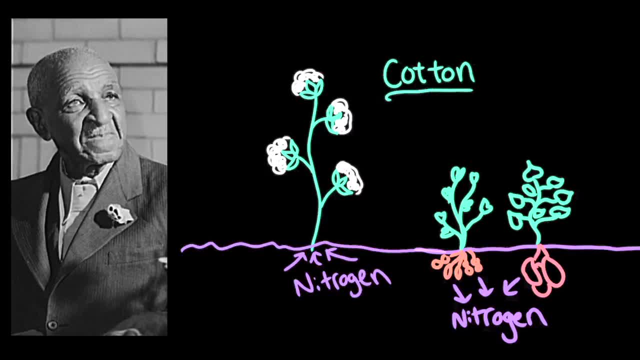 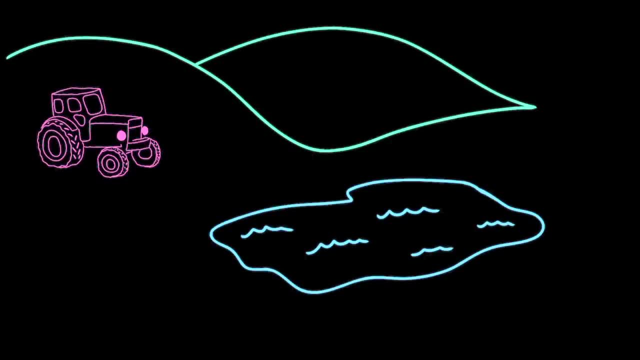 nitrogen back into the soil using chemically synthesized fertilizers. But sustainability is more complicated than just replacing depleted resources. When farmers use too much fertilizer or use poor methods of fertilizer application, all that fertilizer can run off into neighboring waterways. This excess nitrogen in the water could cause a lot of algae to grow. The thing about algae. 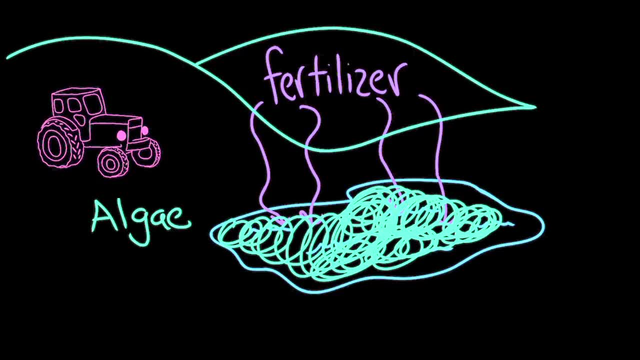 is that when it grows too much, it can cause a lot of algae to grow. When it grows too much, it can die too rapidly and the microbes that decompose the algae hog the available oxygen in the water, which makes it difficult for other organisms living in the water to breathe. So when the fertilizer 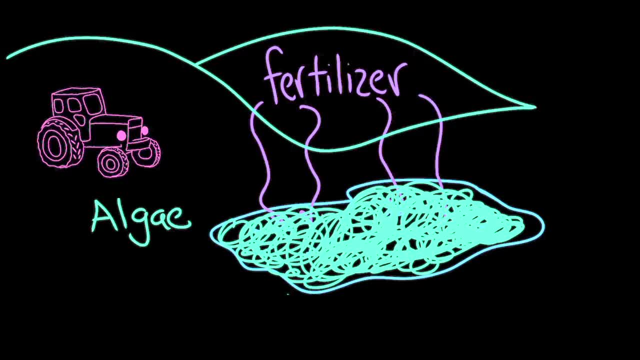 runoff causes too much algae to grow. it creates an imbalance in the ecosystem and harms the other organisms that rely on the dissolved oxygen in the water. So the addition of too much fertilizer is also unsustainable. But how could a farmer know whether they're using fertilizer sustainably? 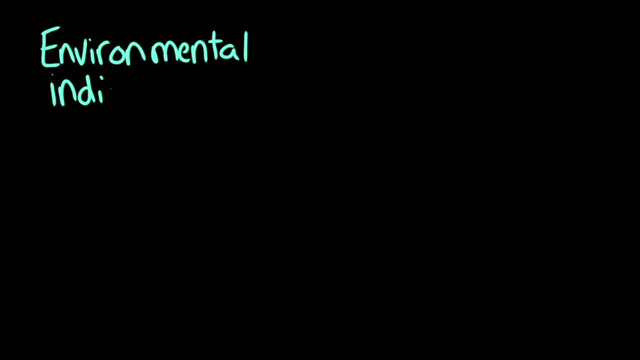 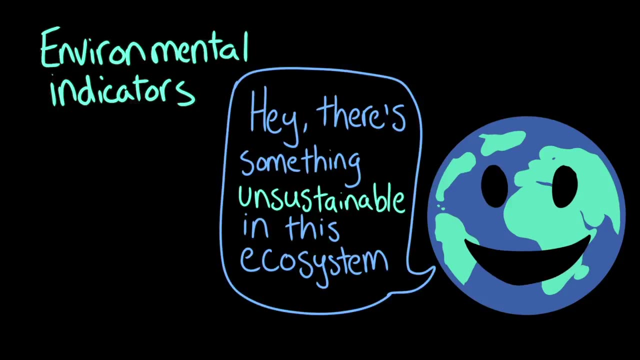 Well, they could look out for environmental indicators. Environmental indicators are basically when the earth tells us, hey, there's something unsustainable in this ecosystem. But instead of just telling us that straight out, it tells us in a variety of clues For our farmer. 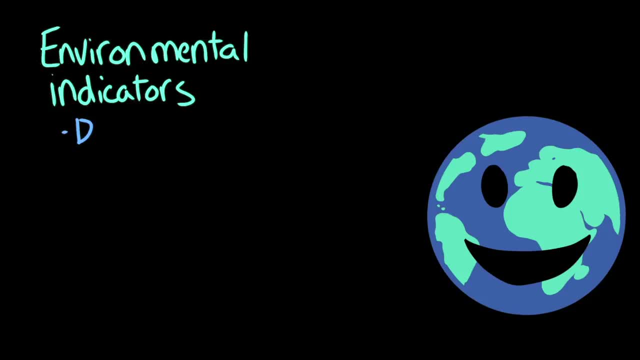 environmental indicators can be things like the amount of dissolved oxygen in the water, the biological diversity in the area or even how much algae grows in nearby water sources. The series of species that are native to nature can direct the water in some way, so they're known to survive. 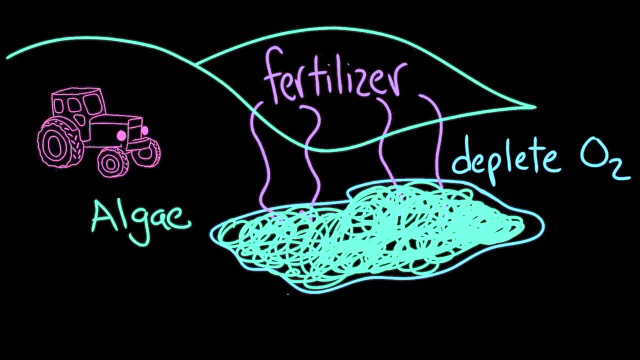 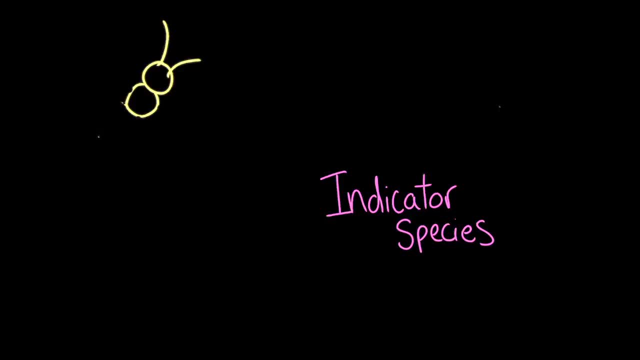 in very specific circumstances. These are larger species that live in the water that require a lot of oxygen to survive, And this is why we've started to call them indicator species, because they're known to survive in very specific circumstances. Spotting these species is. 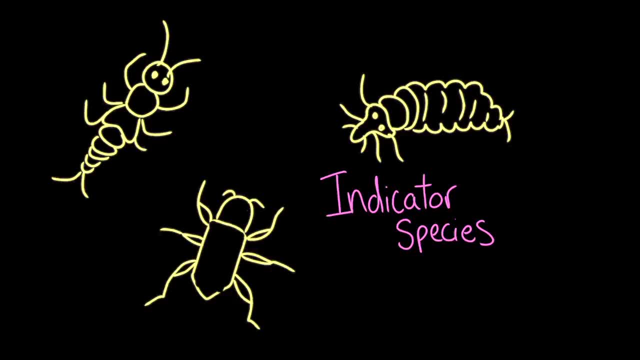 an indication that there is a lot of oxygen in the water. If these species are absent, then that will be an indication that the pollution has reduced the amount of dissolved oxygen in the water- oxygen in the pond. The farmer could then change their behavior In this way. environmental. 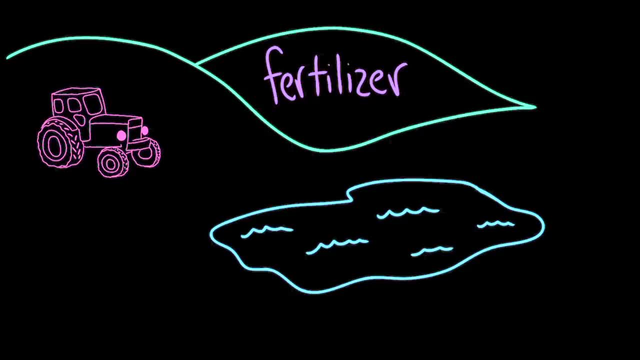 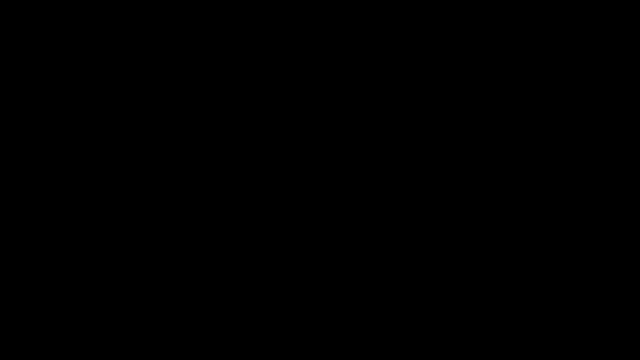 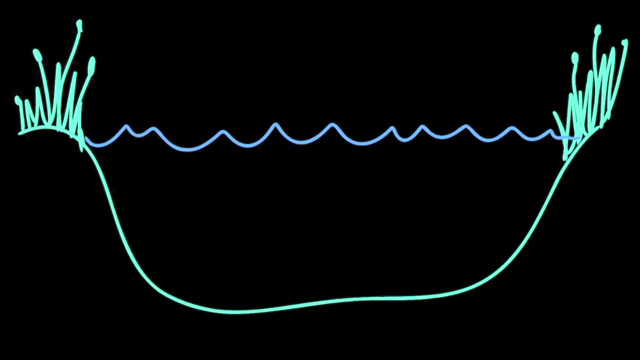 indicators can guide humans to make sustainable choices. Another way humans can use environmental indicators to make decisions about natural resources is by monitoring populations and estimating their growth. Imagine that you have a pond in your backyard and let's imagine that you have searched for all the correct environmental indicators so you know that the fish in your pond 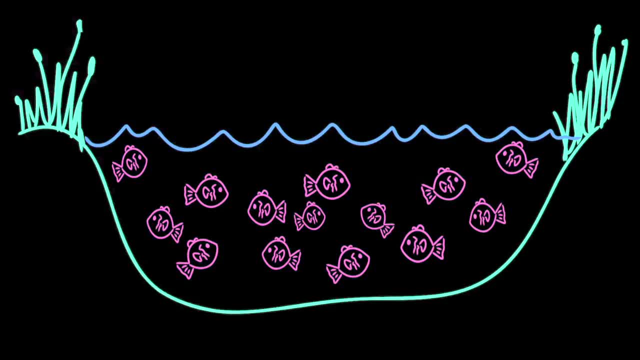 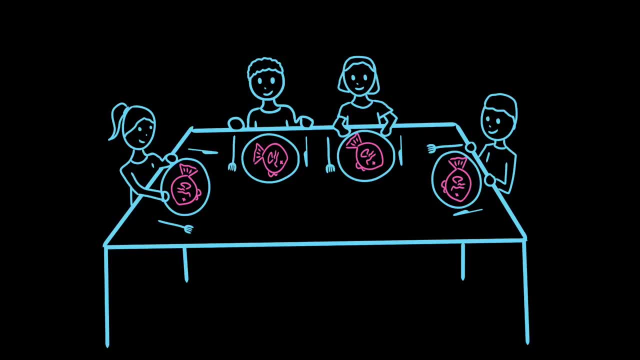 are not suffering from pollution. One day you decide to go fishing. It might be tempting to fish as much as you can so that you can invite all your friends and have a big happy fish feast. But if you decided to take all of the fish out of the pond then there wouldn't be any left to. 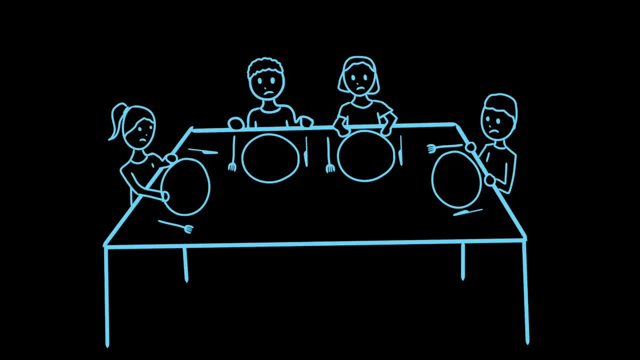 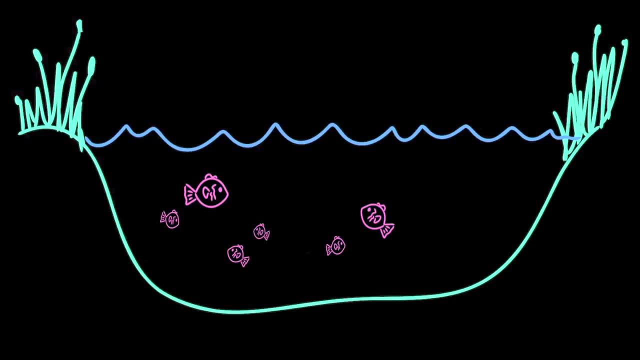 reproduce, so your feast next year would be pretty sad. Even if you just left a couple of fish in the pool, they might not be able to reproduce enough to replenish the population. Other environmental factors might cause the small fish population to go down even further. 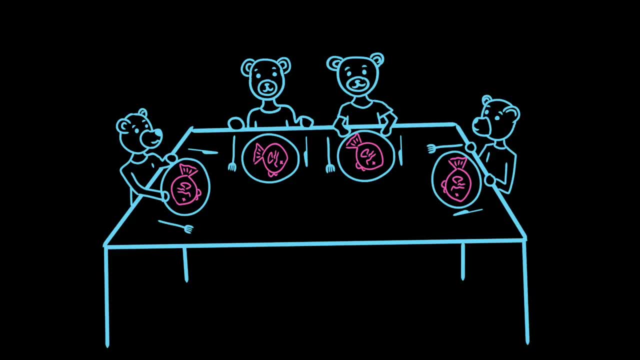 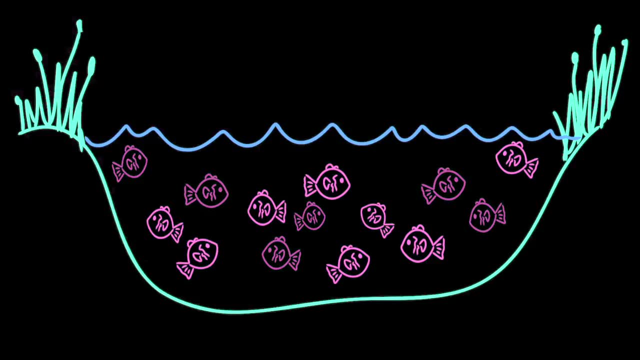 The fish might catch diseases, run out of food or end up being some other creature's feast. There's some maximum number of fish that you could take so that there's enough fish left in the pond to reproduce and replenish the population. This number is called the maximum sustainable.